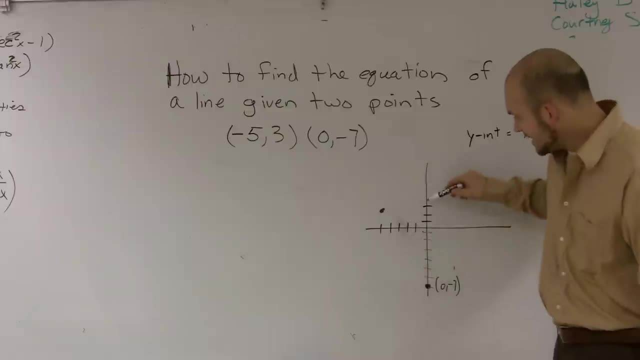 to right. I have to go over 1,, 2,, 3,, 4,, 5, and then I have to go down negative 10.. So I could say the slope is over 5, down negative 10,, which is a negative 10.. So I could say: 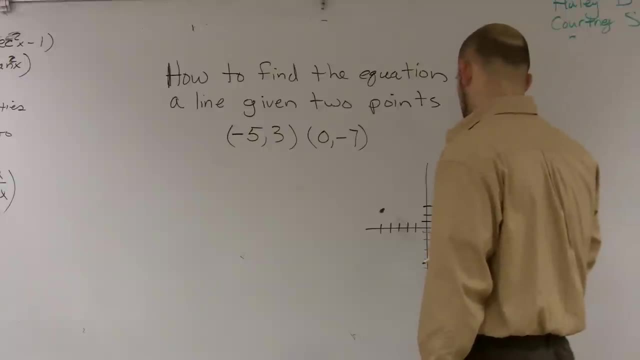 slope to the right change in rise over. run other way. Slope is your change in y, which is down. how far? Which would be down 10, over 5, to the right 5, which is a negative 2 over. 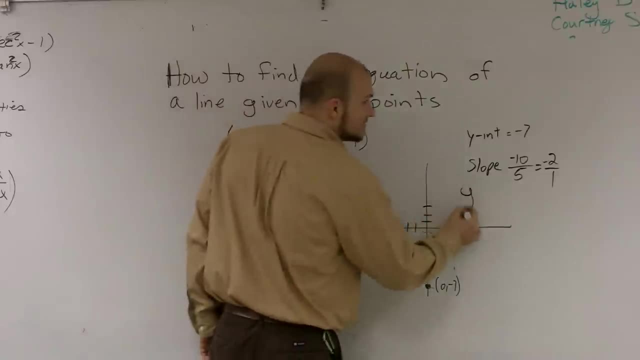 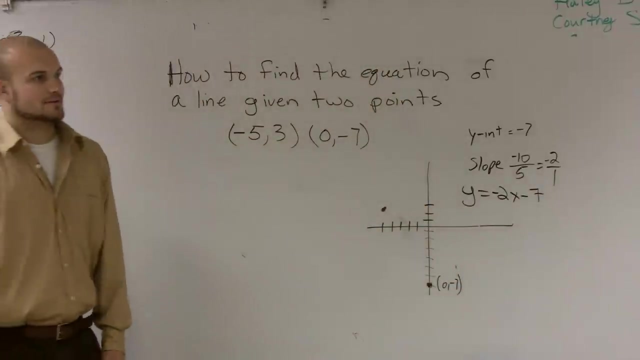 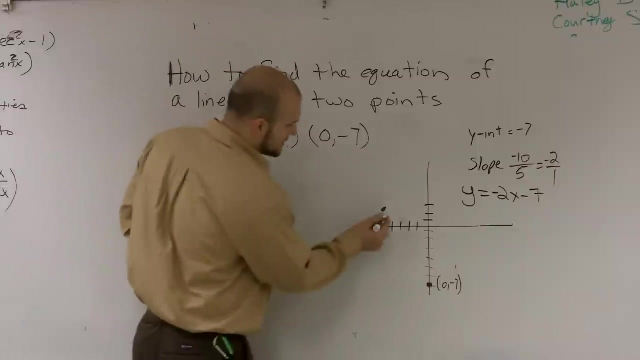 1. There you go. So, essentially, if I want to write the equation, I'm going to show what the answer is. y equals a negative 2x minus 7.. OK, Yes, Thank you. So if I was just going to do this on the graph, I could find out what. 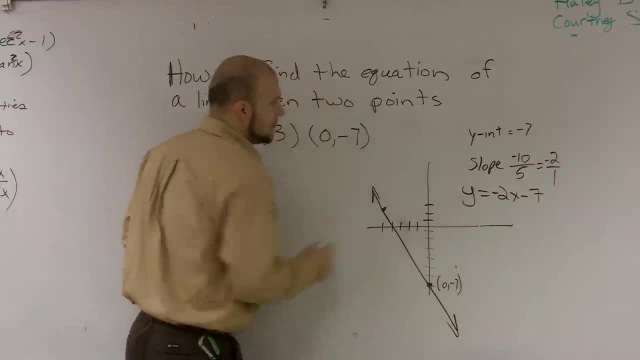 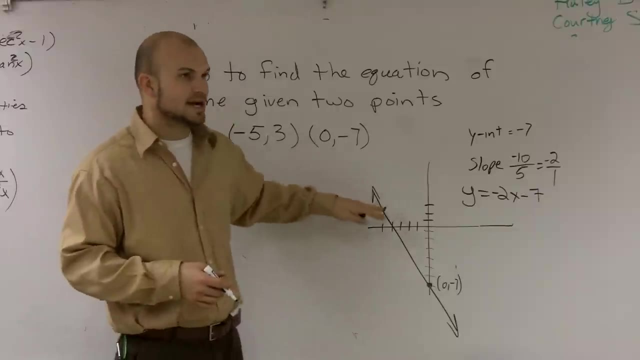 the equation was. However, we're not asking this, We're asking: I want to show you guys a way, algebraically, to find it. So a lot of times you're not going to have something that's easy to graph, so you're going to have to use algebraic methods. So the first method, 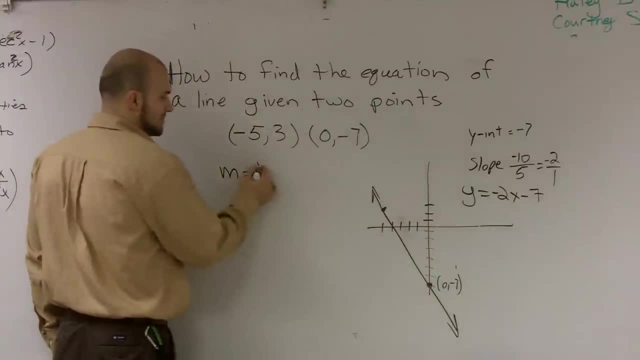 I'm going to show you in this video is using the slope formula which we completed before, which was y1 minus 7.. Y2 minus y1, and x2 minus x1.. So when I want to find the slope between these two points, 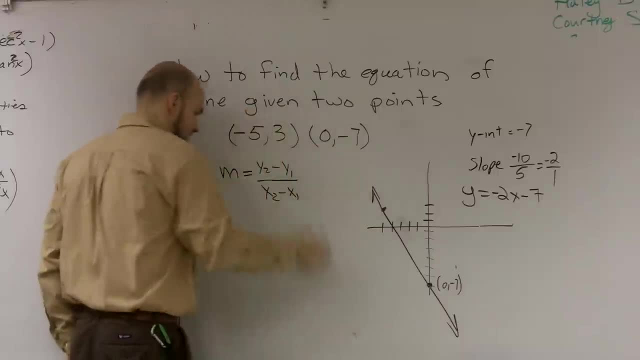 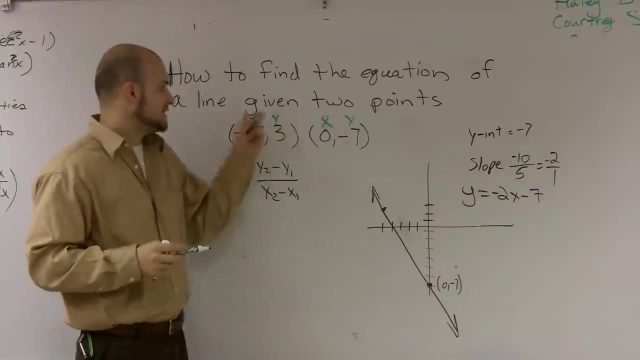 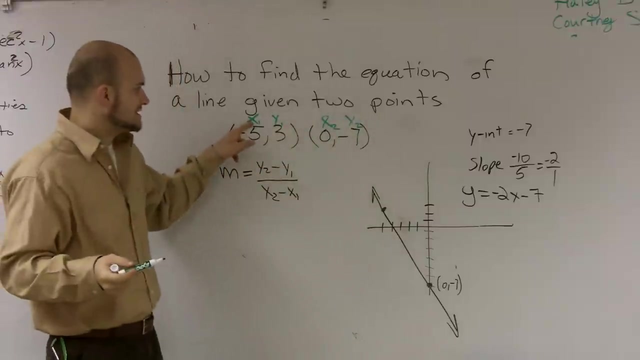 I'm given two points. Now remember each point has a coordinate- x and y- And the way that we like to differentiate between our x's is we just give them little subscripts. It really means nothing more than just saying this x is different from that x. They're both x's. 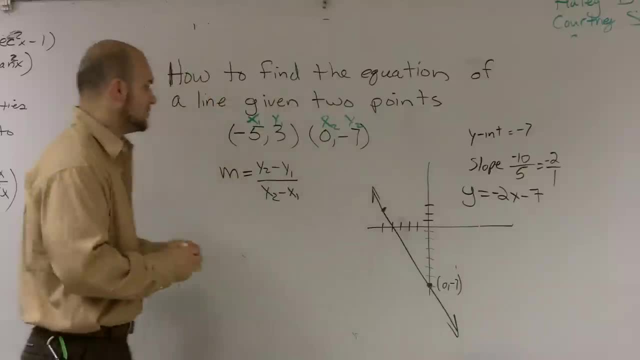 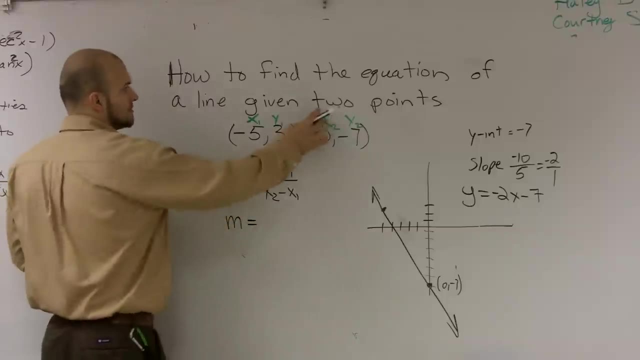 but they're just different coordinates. Right, they're different points. So all I do is I plug this into my formula to find my y-intercept. So what I'm going to do is I'm plugging my y-intercept, which is our.